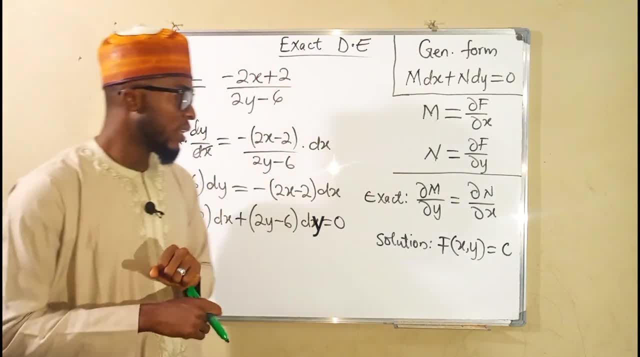 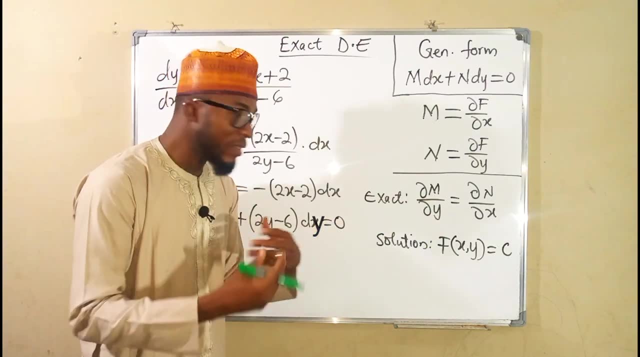 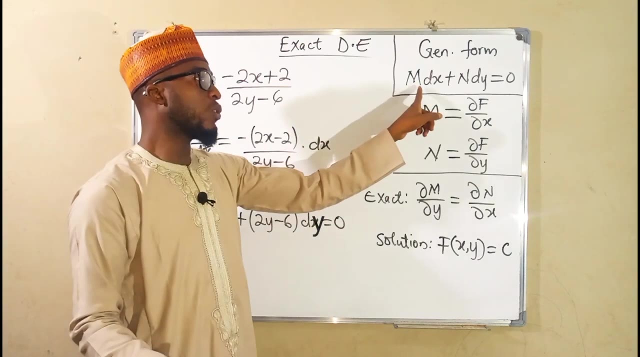 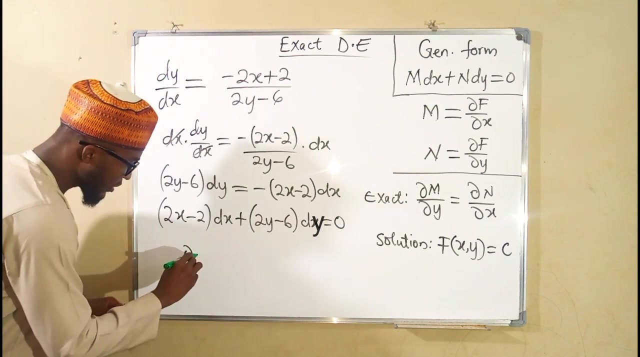 have to do next is to test whether it is really exact. to find out, we have to take the partial derivative of M with respect to y and see whether it is exactly the same as the derivative of n with respect to X. our M is the term which is connected to dx, which we have here, so the partial derivative of M. 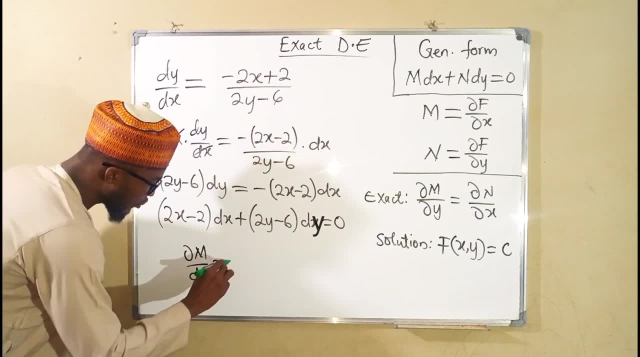 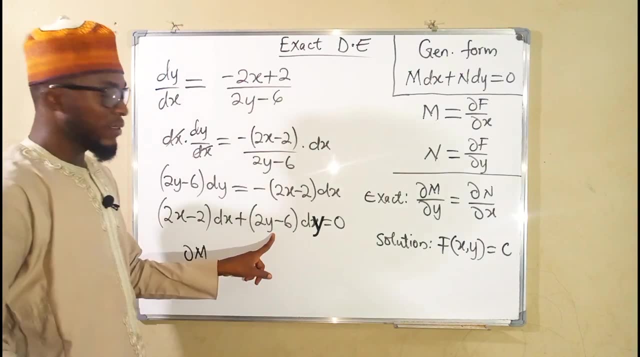 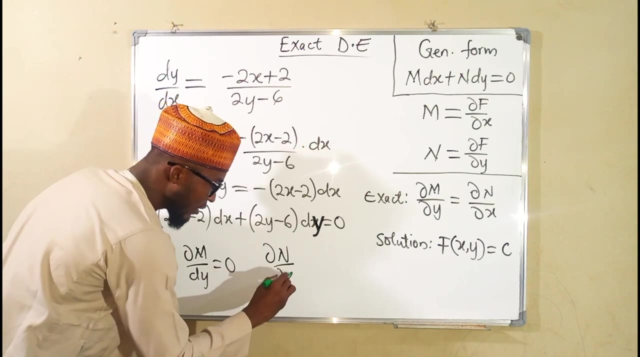 with respect to y is equal to 0 because we do not have any term written in terms of y, then n is this time which is connected to dy. so the partial derivative of n with respect to X is also equal to 0 because we do not have any time written. 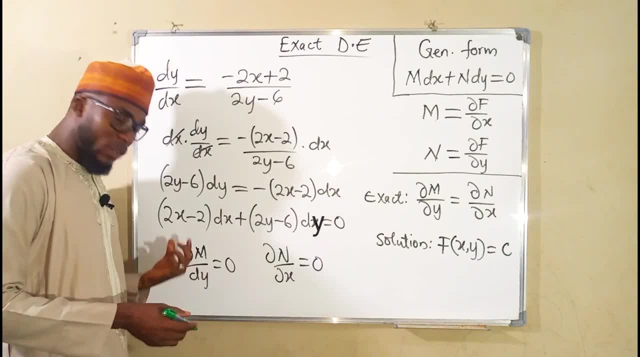 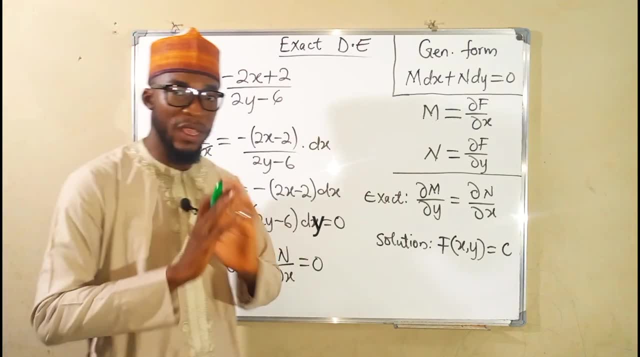 in terms of X here. so you can see, the partial derivative of M with respect to y is the same thing as the partial derivative of n with respect to X. hence we say: the equation is exact. so now let us find out how we can find the solution. 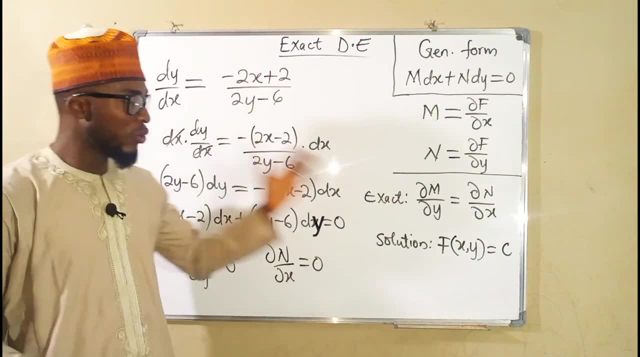 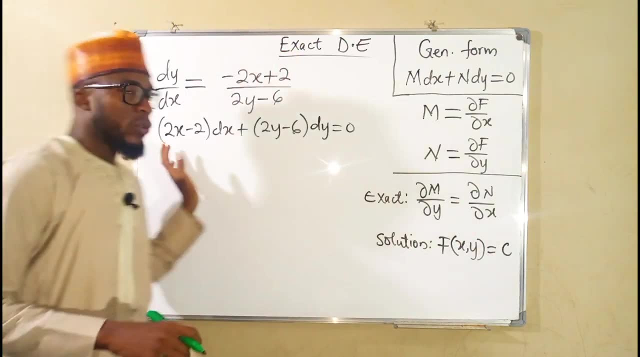 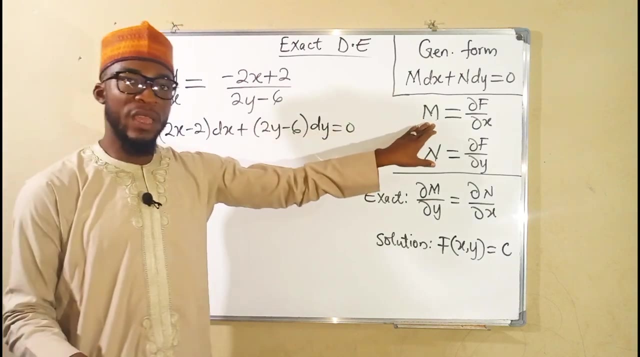 to this problem. the solution to this problem is going to be in the form of F, which is the function of x and y, equal to some certain constant. so now, this is the differential equation we want to solve: the time, which is connected to dx. you know, we say it is M, and M is the partial derivative of f. 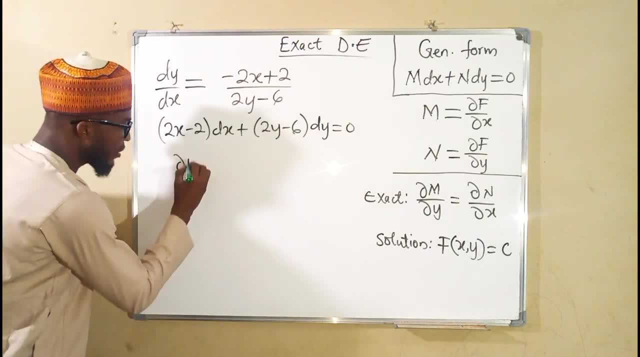 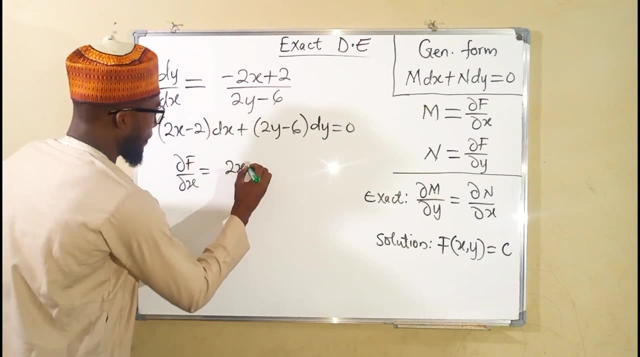 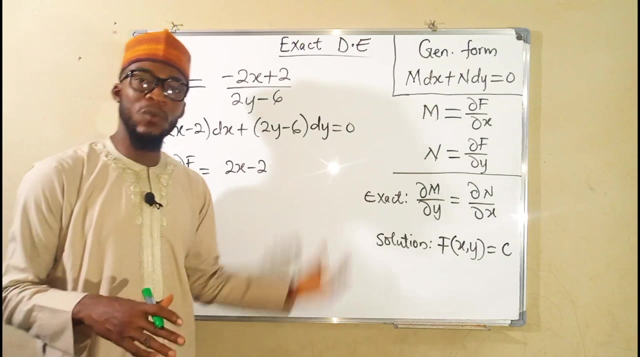 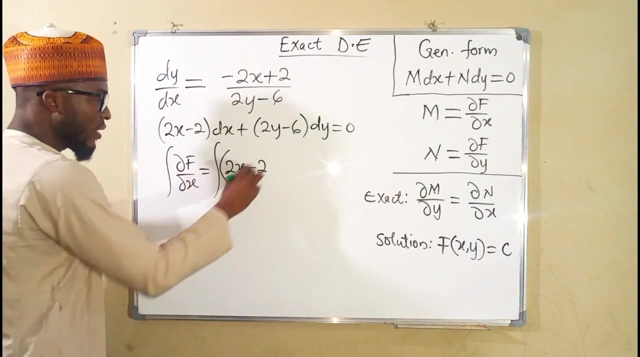 which respect to X. so we see, the partial derivative of f with respect to X is equal to 2x minus 2.. Now we want to solve for f, which is a function of x and y. We are going to integrate both sides with respect to x, Integrate this side, integrate the other side with respect to 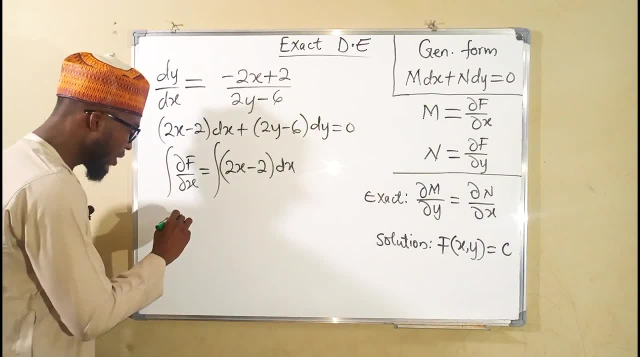 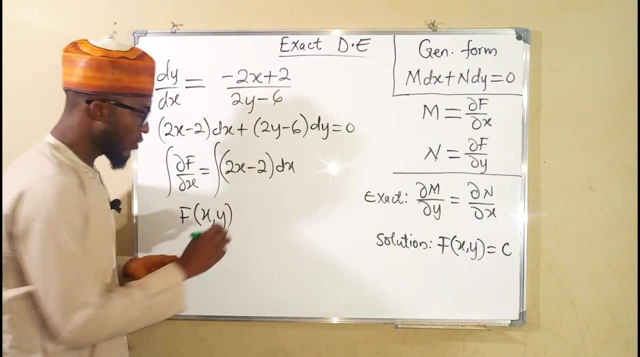 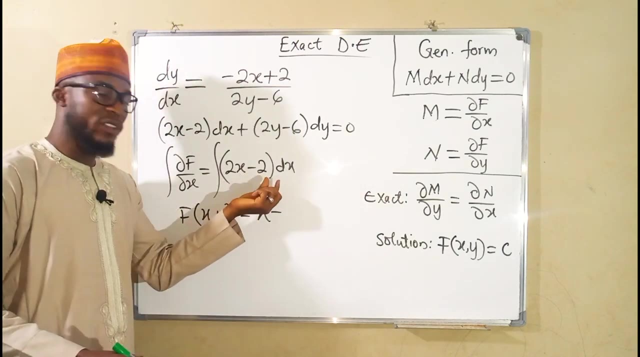 x. Integrating the left hand side, we will be only left with f, and this f is a function of x and y. And to the right, if you integrate 2x, you are going to obtain x squared minus. if you integrate 2 with respect to x, you are going to obtain 2x plus our constant of integration. 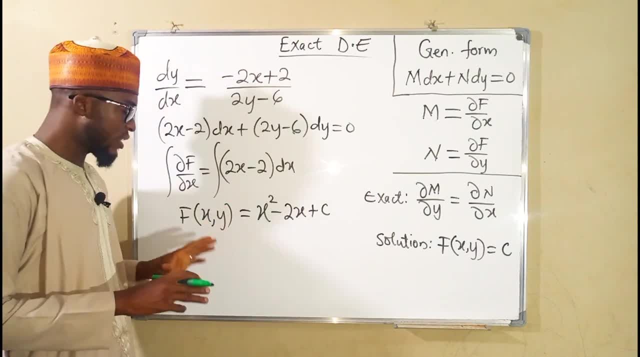 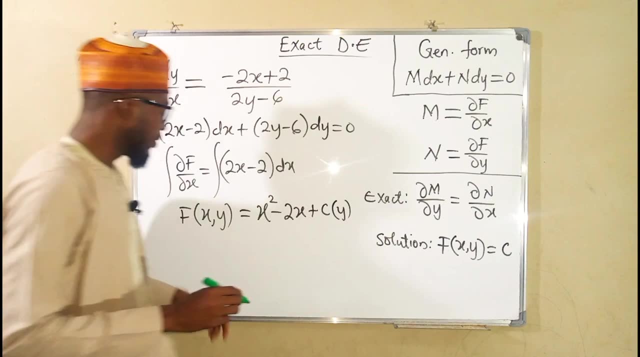 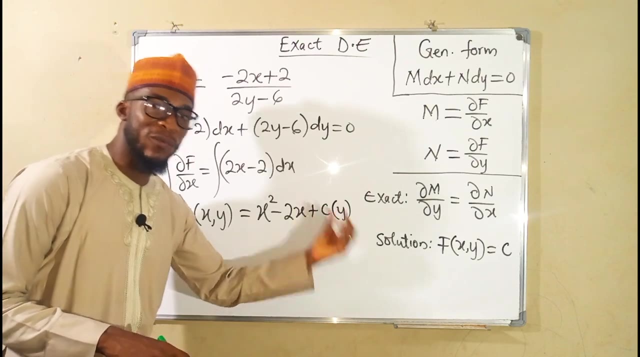 But remember, this is an implicit function where we treated y as constant. therefore our constant is going to be in term of y, So we have c of y here. So this is our solution to this differential equation. But we have to find the real value of this c of y. 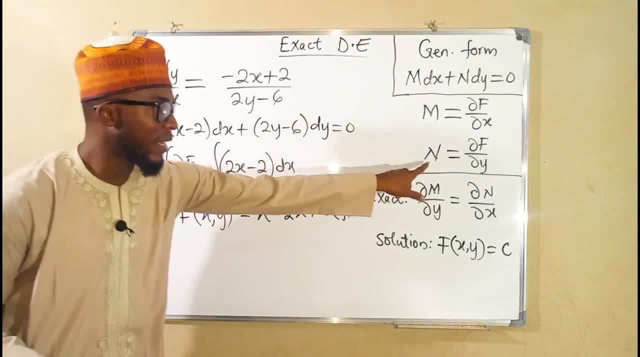 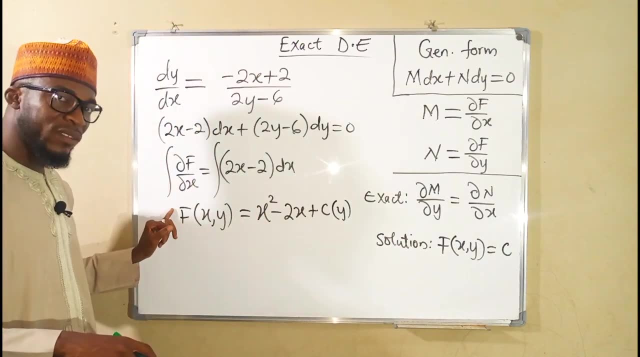 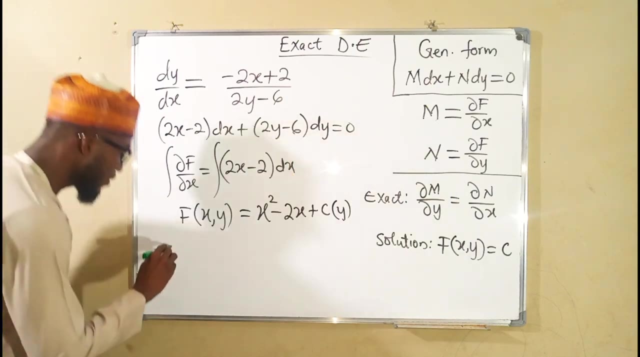 Remember the term which is connected to dy. we say it is n and n is the partial derivative of f with respect to y. Therefore, we can differentiate this with respect to y. Whatever we obtain here, we are going to relate it to this. So we say the partial derivative of f with respect to y. 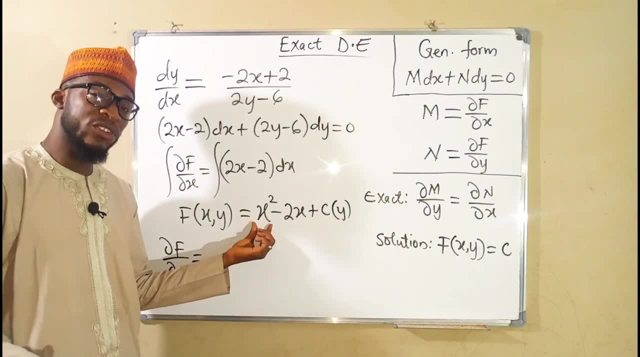 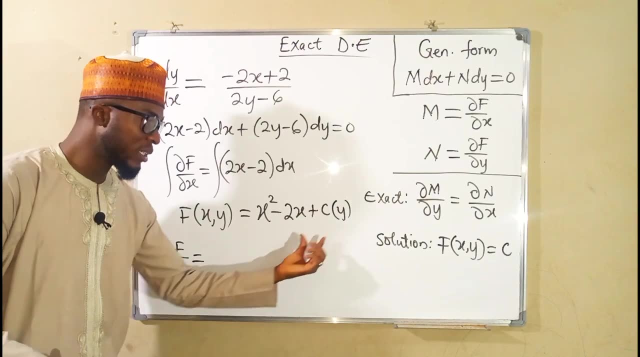 Here you can see that what we had obtained is equal to will be: the partial derivative of f with respect to y will be reflected on the derivative c of x, plus the difference of the 2 is equal to x. we are going to treat it as constant, therefore. 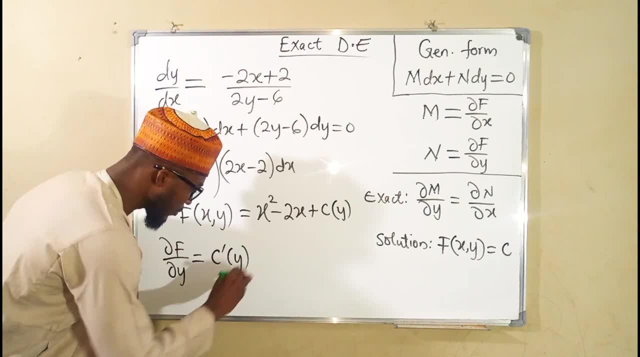 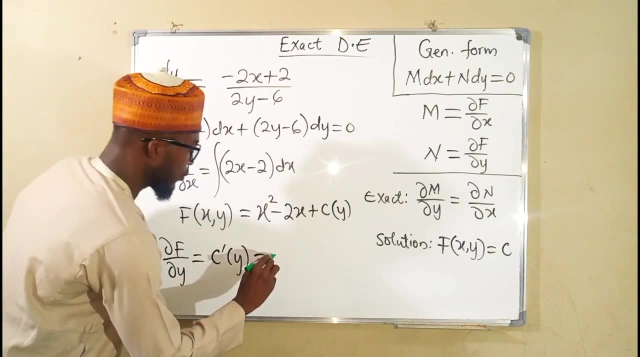 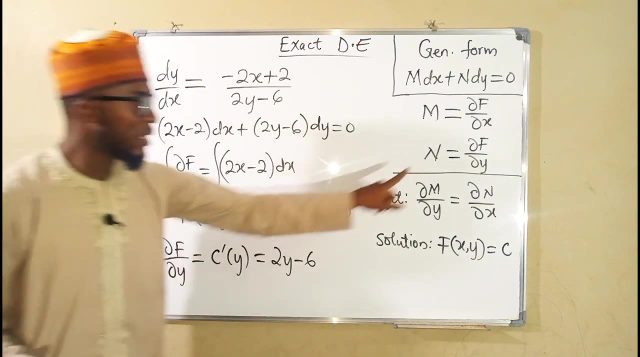 we have zero here. we have zero here and this is c prime of y. so we only have c prime of y here. This c prime of y must be equal to two y minus six, because we say respect to y is n and our n is 2y minus 6.. But we are looking for c of y, not c. 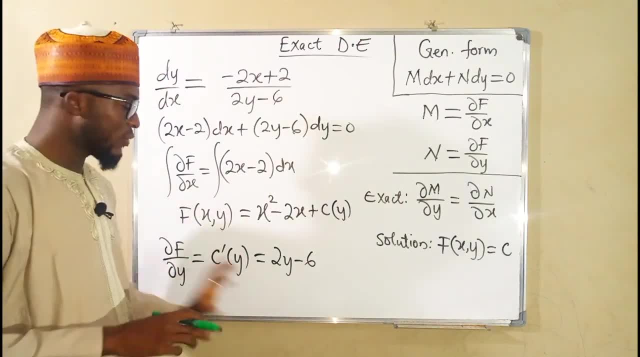 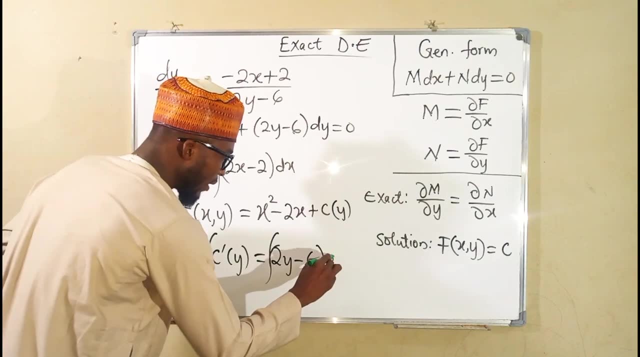 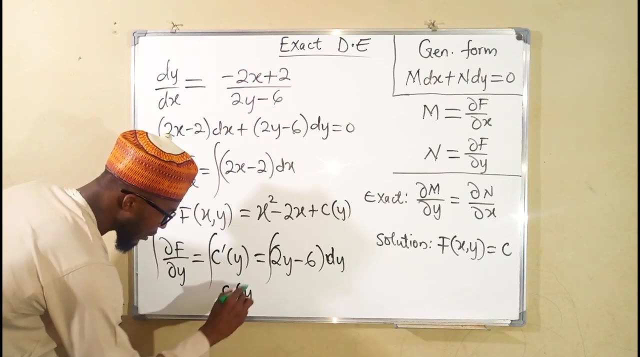 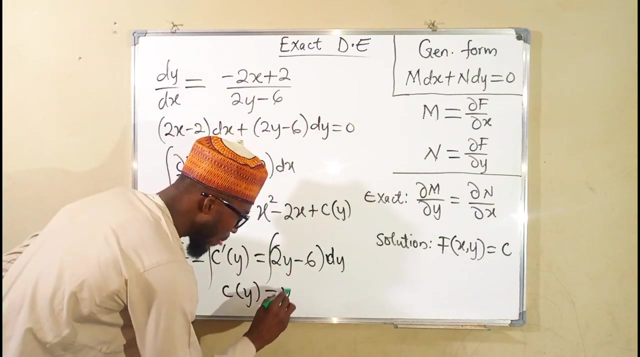 prime of y. Therefore, we can integrate both sides with respect to y. So we integrate this with respect to y. This becomes only c of y. This is equal to: if you integrate to it with respect to y, you're going to obtain y squared minus. 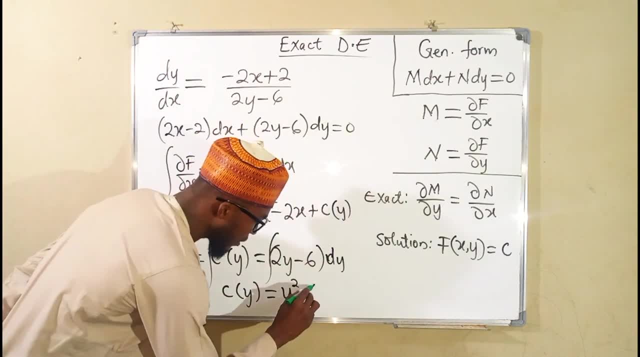 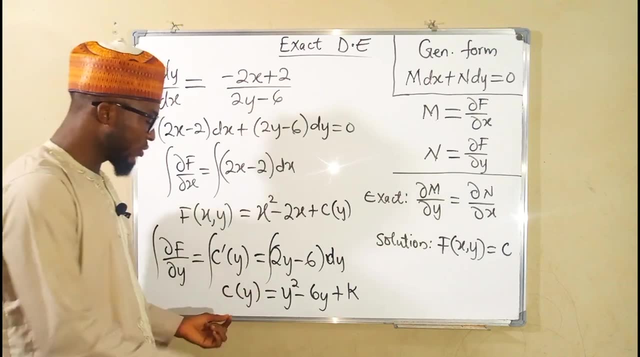 integrate six with respect to y, you're going to obtain 6y plus constant of integration This time around. this is not implicit function. it's a function with respect to only y. So we have now obtained c of y, which we are going to substitute. 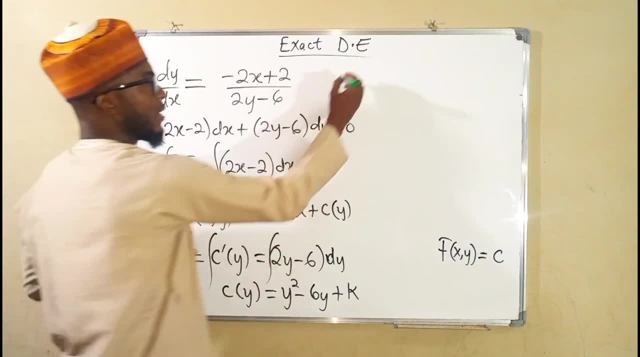 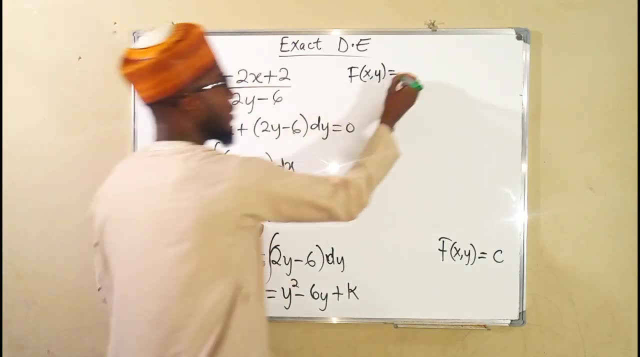 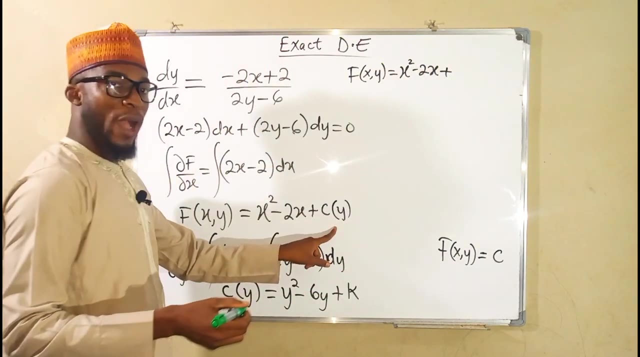 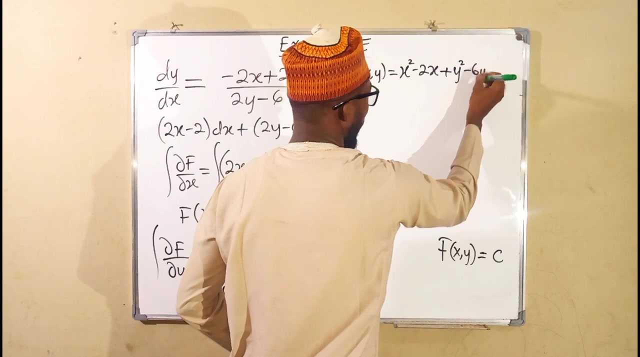 here to obtain our general solution. So finally, we have a function of x andamı y equals. we have x squared minus 2x plus c of y, but c of y is y squared minus 6, y plus k, y squared minus 6, y plus k. but our real solution is going to be a.